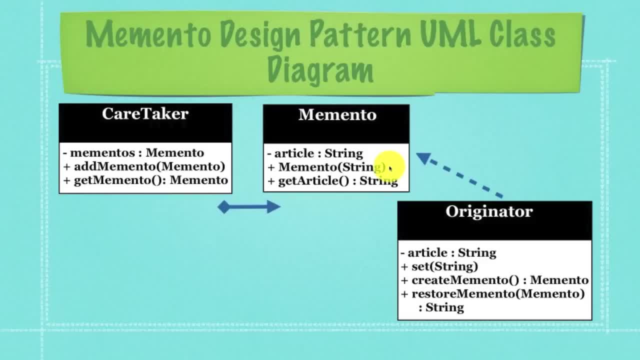 memento. Memento, of course, is going to be the constructor which is going to create a new memento object with a new article stored in a field, and then you're going to have get saved article which is going to return the value currently set for the article, which is right here. Then let's jump over to the 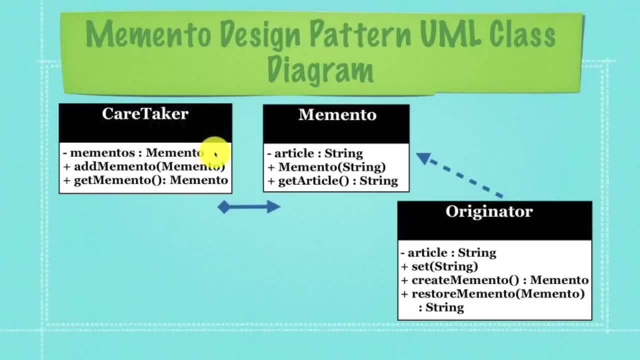 caretaker. First you're going to have an array list of memento objects. Then you're going to have the ability to add memento objects to the array list as well as get objects from that same exact array list. You have the originator. We're going to store a value for article inside of it. Set is going. 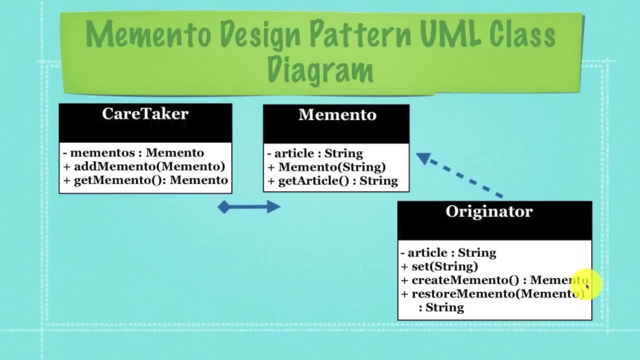 to create a new article field. Create memento is going to create a new memento object, which it's going to do by sending a new article field to it. See, that's what this string is: the article field. Then, finally, you have restore from memento, which gets the values of article for the current. 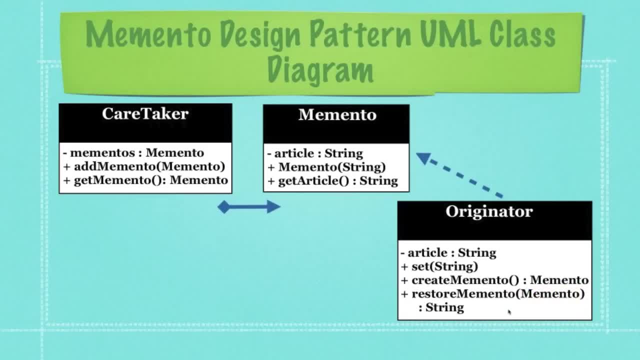 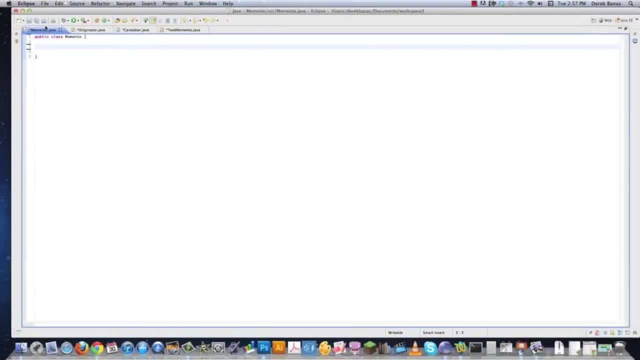 memento object that is set. So there is a brief overview, as well as a kind of uml class diagram. So now let's jump into the code and explain it further. Alright, so here's everything. The first thing we're going to do is create mementojava, which is going to be the objects that we're going. 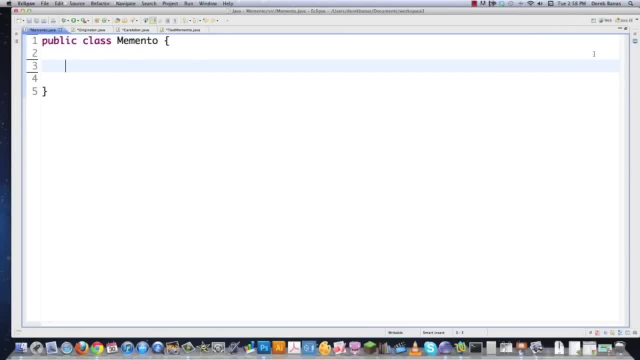 to be storing, and there, everything is on the screen. The first thing we got to do is create the article that's going to be stored, the memento object. I'm going to make this a private string and I'm going to call it article. and then I'm going to create a constructor memento. that's: 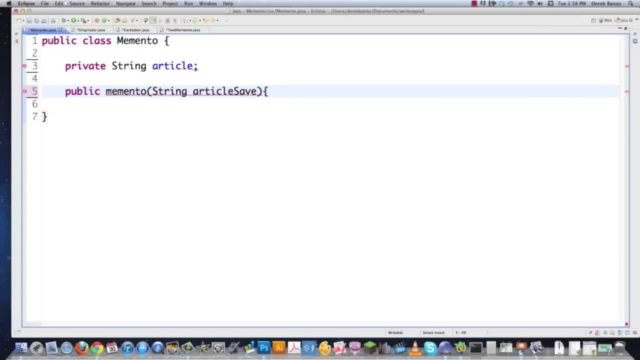 going to be passed an article that's going to be attached to it, article save, which is going to be stored in here and there you go and, of course, make this capitalized and then, finally, we need the capability to return the value stored in the article. So we're going to go public string get. 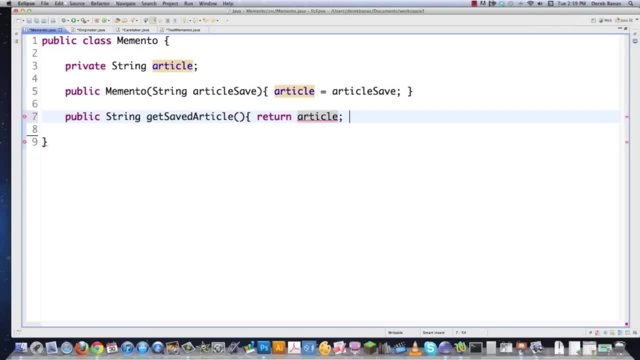 saved article and, quite simply, it's just going to return the article field value for said memento and that is it. So there is the memento and, as you can see, it's really simple. I just have the article saving here, but you can have numerous different fields saved and, of course, you could. 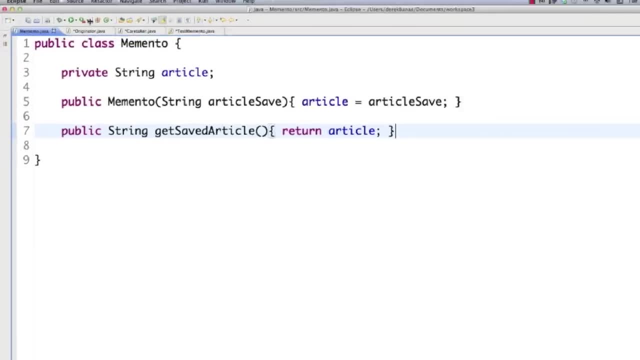 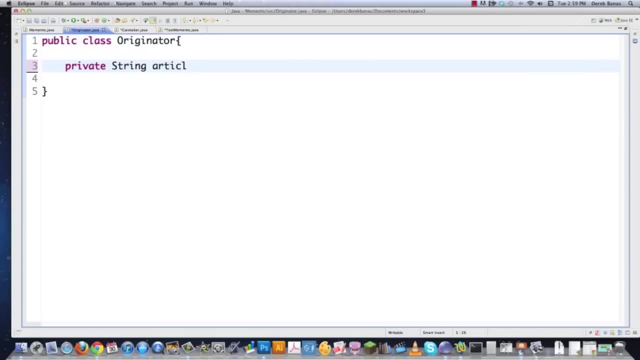 use composition to have multiple different objects stored inside of it. So now let's go into the originator and see how this guy's all created. We're going to have private string which is going to be a temporary holding cell for whatever is going to be stored in article, and then we're 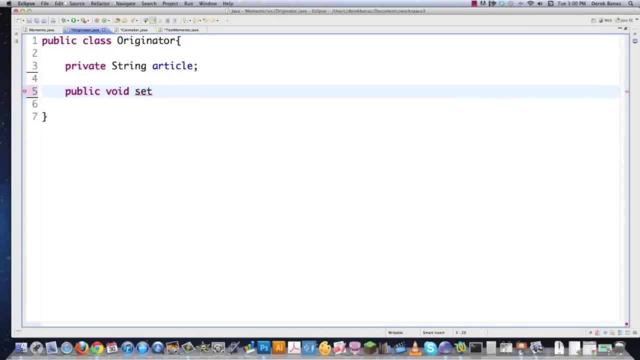 going to go public void set, which is going to set the value for our article, So a string is going to be passed over to it and then, so we can track everything, I'm going to print different messages out on the screen, and all this code is available underneath the video, and you should definitely 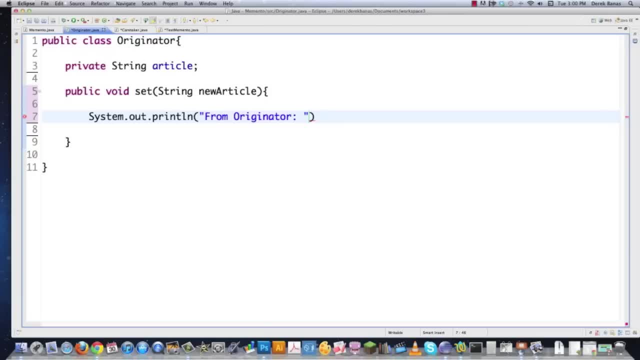 download it and play around with it if you really want to understand how this is going to work. So now I'm going to go to the project and I'm going to create a new version of article, throw a new line inside of there and then I'm just going to go new article so that we'll be able to figure out. 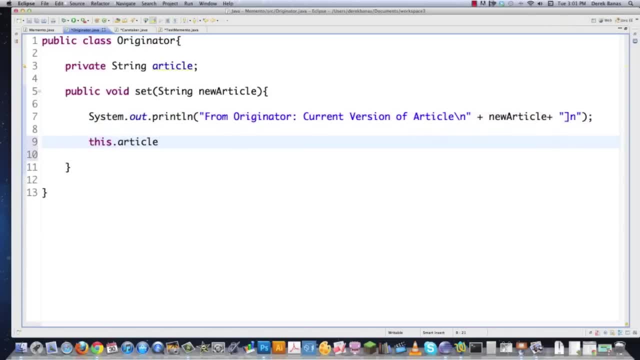 exactly when changes are being made to it. Okay, so we got that all set up and then I'm just going to go. this article is equal to. actually, I don't even need the this part here, I can just go: article new, article. Alright, so we got that saved. then we need to create a new memento with a new article. we're. 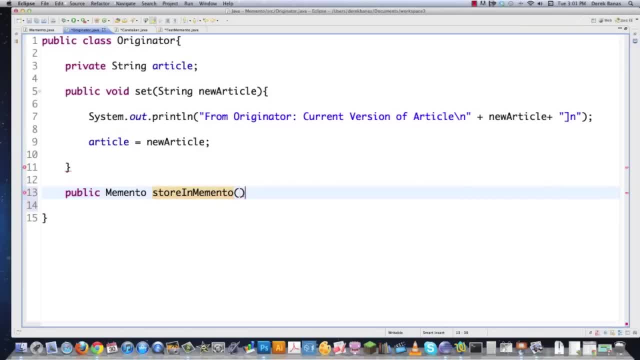 just going to go. it's going to return a memento object- It's going to be the name of this method- and then we're also going to print out another message on the screen so we'll be able to track what's going on with this. and I'm just going to say from. 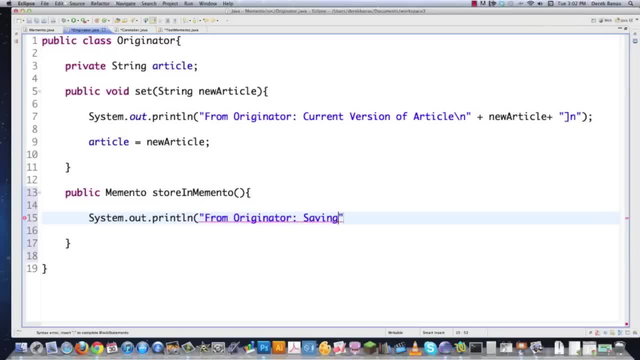 originator, so that you'll be able to see where that's going. saving to memento blows that off and then we're going to return new memento- which is also going to be a call to the memento constructor, of course- which is going to be passed the value that we have set for article. 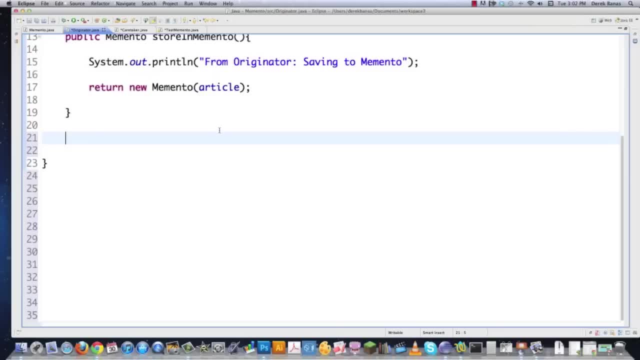 and then we need to get the article that's currently stored in the memento object And we just need to create a new method- I'm going to call this restore from memento- and part of this tutorial is going to be improved and part of it is not, and the reason why is: I wasn't certain if 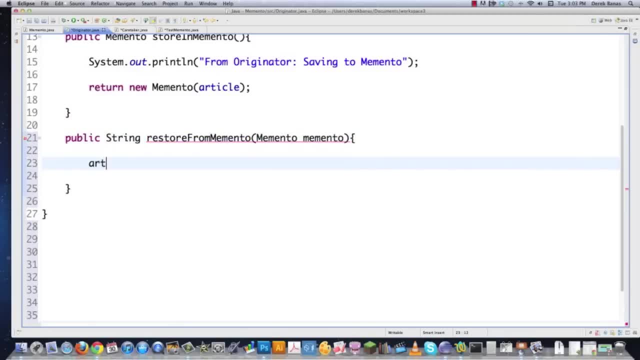 I was going to use any type of swing tools whenever I first started this and now, as I'm doing it, I'm thinking, yeah, I'm going to do it that way. basically, I'm going to allow you to type out an article and then bounce back through previous versions of it and then into future versions of it. I think that's. 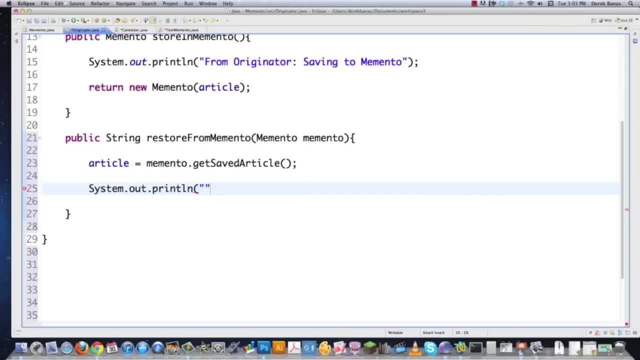 what I'm going to do anyway. See how it turns out: system out print line. and we're also going to go from originator and we're going to put out a message- previous article saved in memento- and then throw another new line inside of there and then print out the article on the screen and then throw another new line inside of. 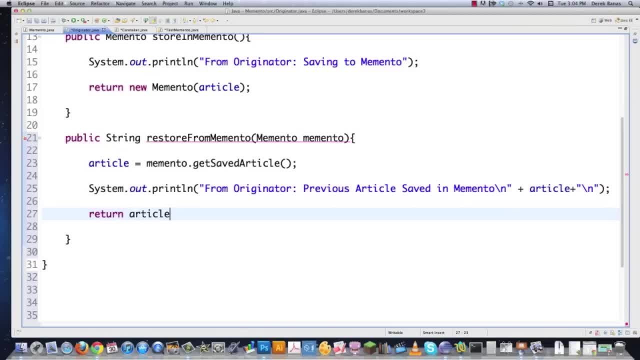 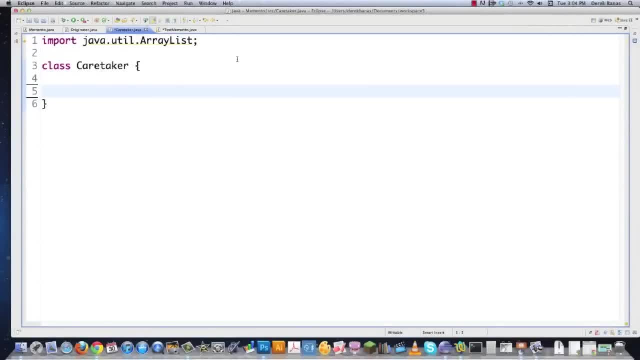 that, and then, finally, of course, we're going to return article, and there we go. so that's all set up, and now we need to go in and create the caretakerjava file, and I already created an array list because I knew that's what's going to be stored inside of here. 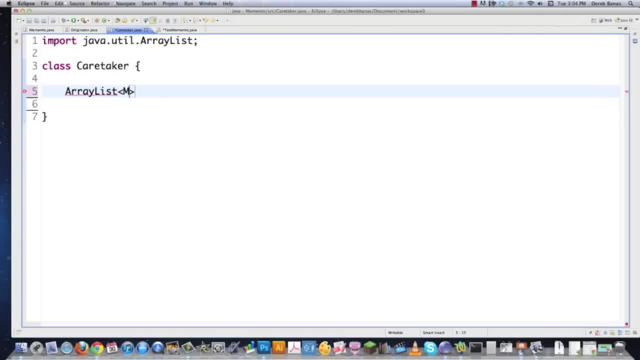 So we need to, of course, create an array list that's going to store memento objects inside of it. saved articles sounds like a good name: array list. memento objects are stored inside of it, and there we go, and now we're just going to manipulate those like we're going to add an article to. 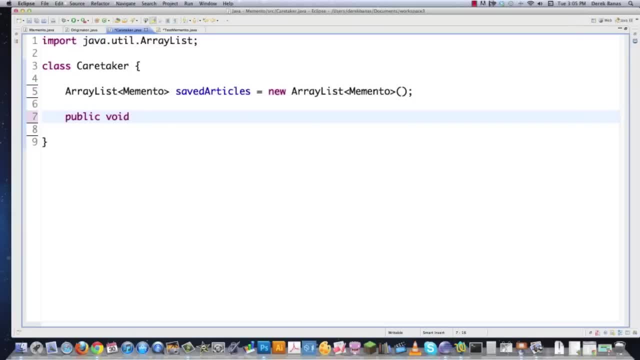 our array list. so let's go public void, where we're going to add a new memento object. I mean to our array list, add memento, and there's the memento we're going to be passing over and I'm just going to create a new table. go save and then prevent type and then save my name and then save articles. 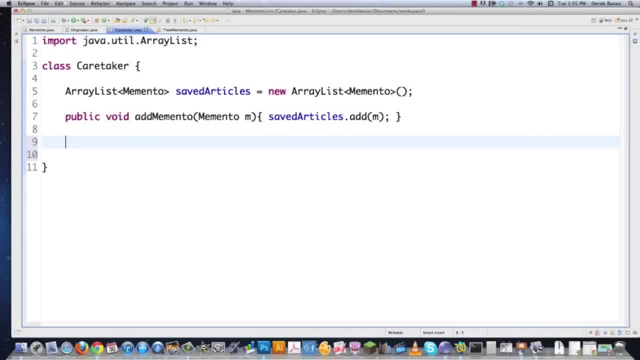 which is actually saved mementos. but whatever you get the point, there we go. that's going to save a new memento, object to our array list and we just need to get those mementos from the array list to do that. we're just going to go public memento, get memento and we're just going to pass an index. 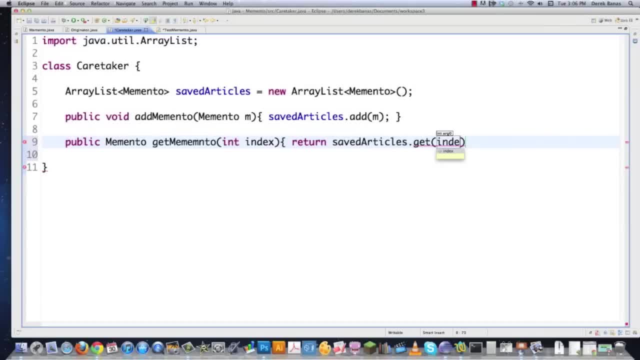 over and that's how it's going to get that requested memento that we want, and then we just have to go saved articles. That's going to get our Memento objects from our ArrayList And there we are. That's pretty much it. 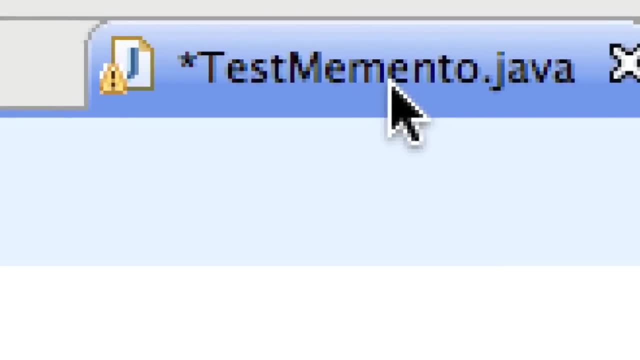 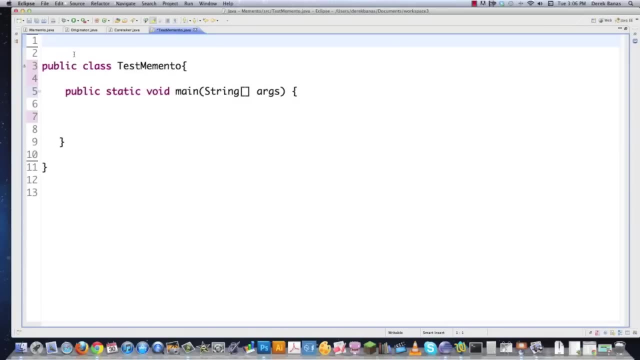 Now that's why I'm doing this a little bit more complicated. Now I'm going to create testMementojava, And this guy is going to use some JFrames and then different swing components to make this a little bit more interesting. So I'm going to need to import some libraries. 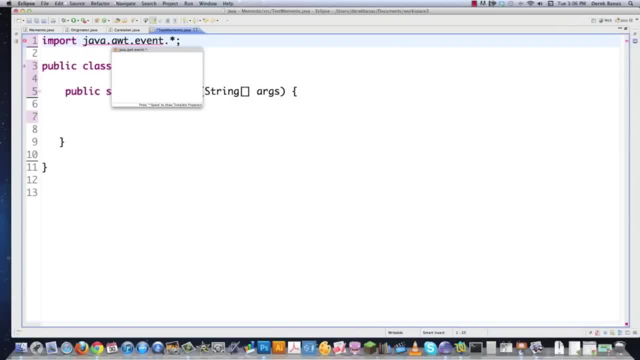 So ought. I'm going to do some event handling So that'll handle that, And then I'm also going to import JavaX swing so that I can use different swing components inside of this, And then if I want to use this as a JFrame, I just need to go extends- JFrame. 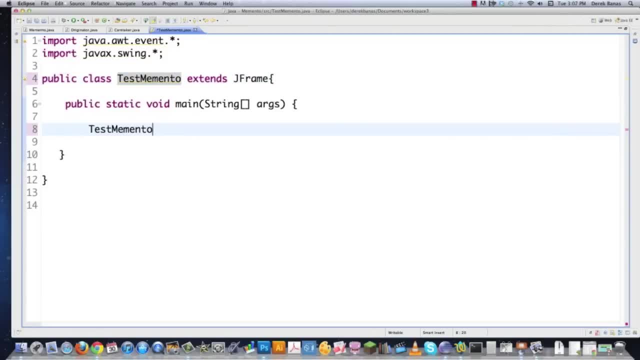 Pretty simple, And then I'm going to go testMemento, Paste that there And then go new. This is going to create our new JFrame that we'll then be playing around with, And then I have to decide exactly what I want to have inside of this guy. 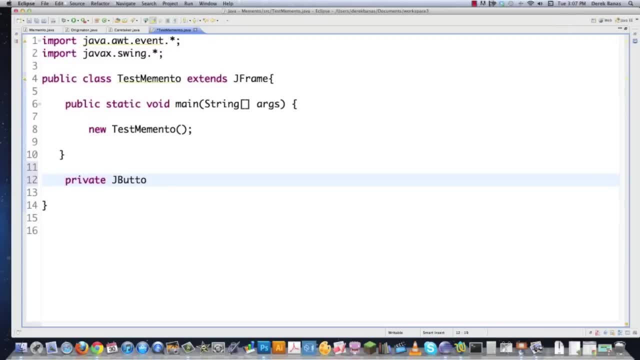 So let's say I want to have private JButton, I want to have some JButtons, I want to be, I want to be able to save my current Memento with the current article that is stored inside of it, And I want to be able to undo. 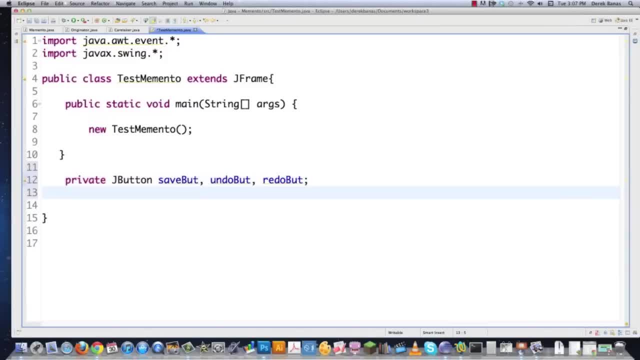 And then I want to also be able to redo So it's going to be able to bounce through different versions of our objects. And then I'm going to go JTextArea And this is just going to be a text area. I'm going to call it the article new JTextArea. 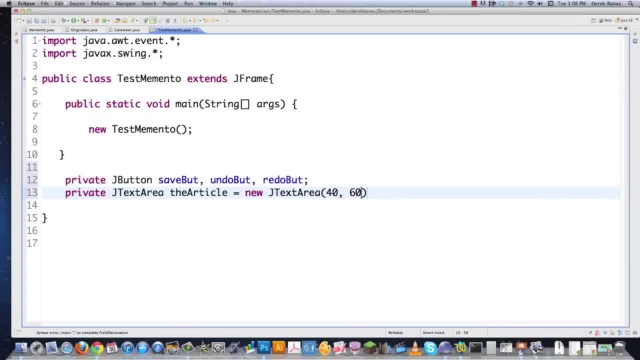 And it's going to be 40 rows by 60 columns. I think that looks about right. And then caretaker- I'm just going to call it caretaker, Is that simple enough? New caretaker And, like I said before, we're going to create the caretaker. 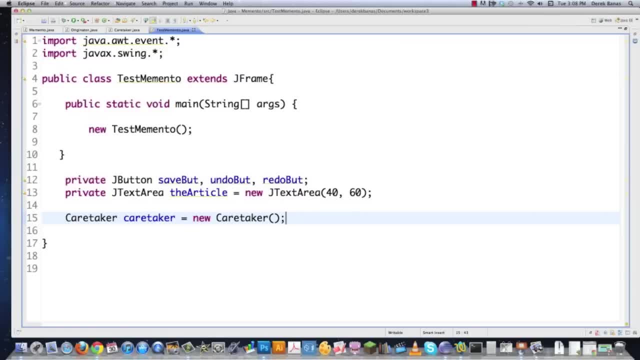 And it's going to contain the array list with all the different Mementos that have all of the different articles inside of it, And it's going to allow us to add and retrieve articles and Mementos from that array list. Pretty simple. 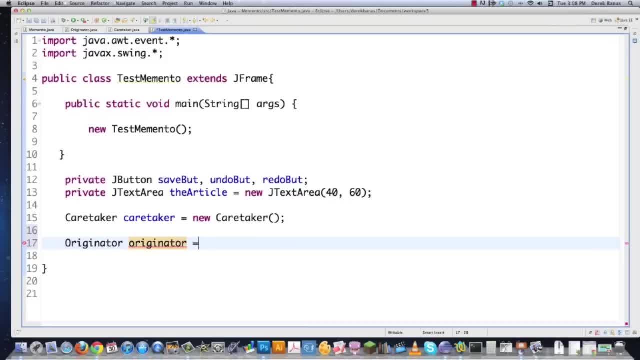 And then we're going to have originator, which I'm just going to call originator is equal to new originator, like that, And the originator is just going to set the values for the article, create new Mementos with new articles and also get the article stored. 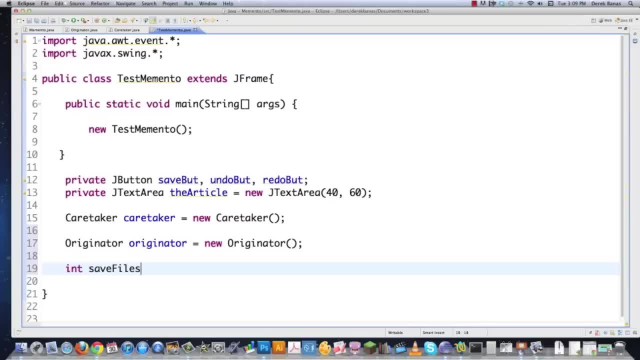 And then I'm going to say save files. which is going to be the number of files that I currently have saved or the number of Mementos I currently have saved? That's going to start out at zero. And then I'm going to say: current article is going to tell me which current Memento 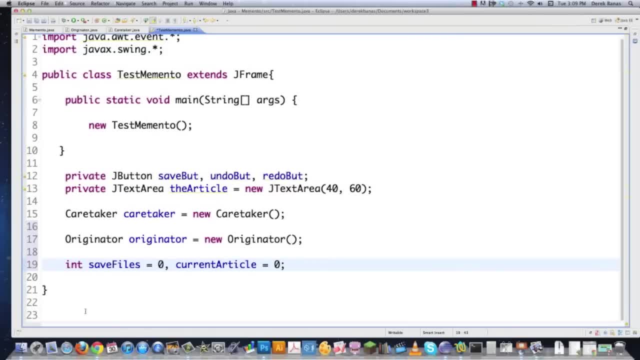 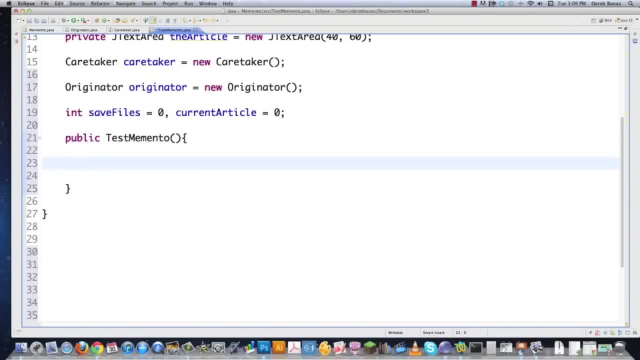 I'm working with so that I pull up the right Memento object whenever I need it, And then public test Memento, which is going to be this J frame. that's going to create everything for us here. Just need to set some basic information for the panel. 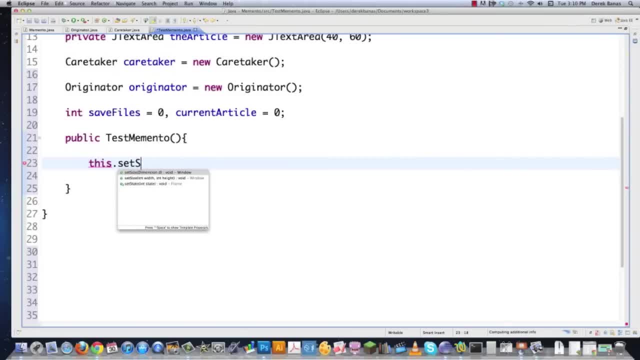 It's going to hold. It's going to hold all of my GUI elements for me. So I'm going to go set size 750 by 780.. It's going to be the size of the J frame, this title, and I'm just going to call this. 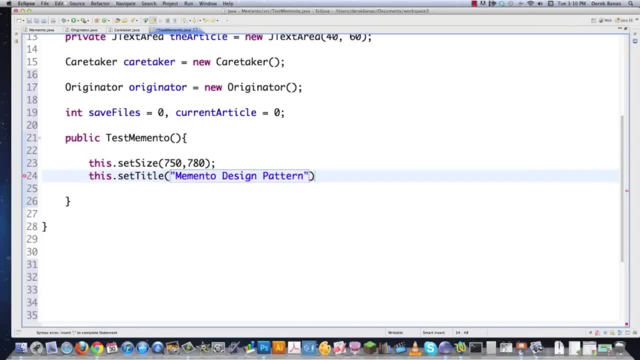 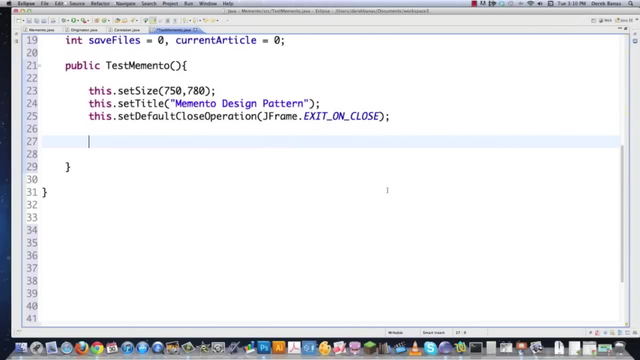 Memento design pattern, because that seems to make sense, doesn't it? And then this also set default close operation. J frame dot exit on close. Sounds like that's going to work good for me, And that's just going to close everything whenever the X button is hit on the J frame. 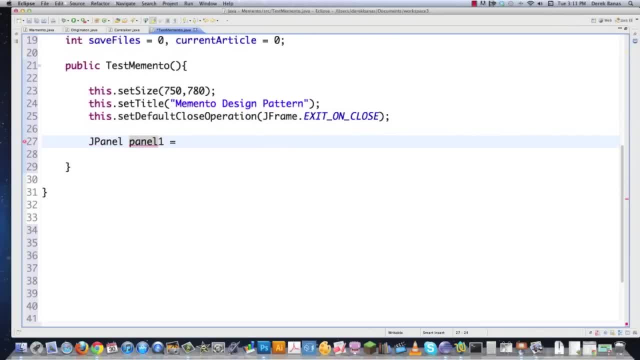 I need to create a J panel which is going to hold all my GUI elements- new J panel. Then I'm going to add a label to my panel, just for the heck of it. So I'm going to go panel one: add new J label. 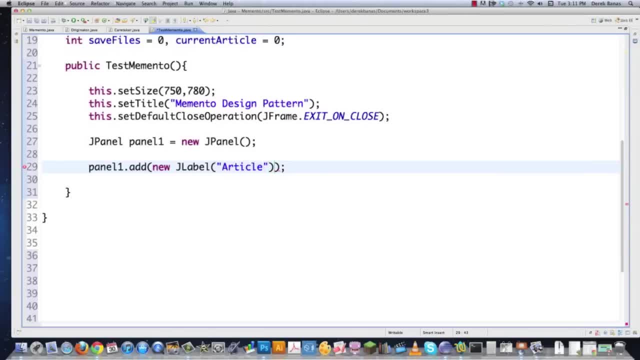 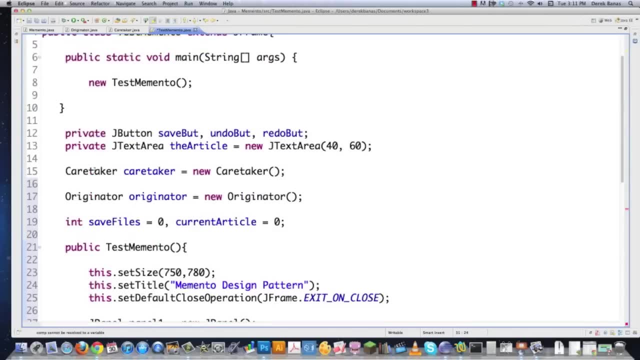 And this is just going to be article, which is going to be the article that's going to be changing and stored and all that other stuff. Panel one: I'm also going to be adding my J panel, or my J text area, which is going 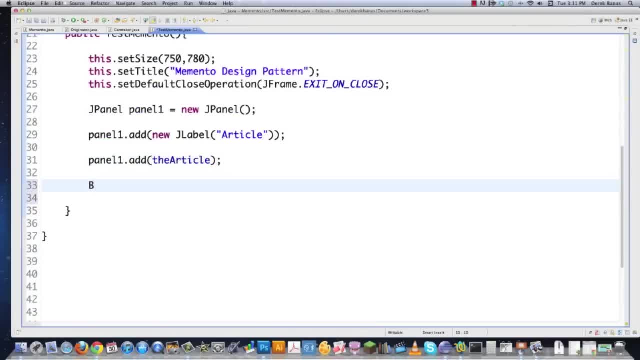 to be called the article. So paste that inside of there And then I'm going to handle all my buttons. So then I can do different things whenever different buttons are hit. I'm going to add little action listeners to this new button listener. 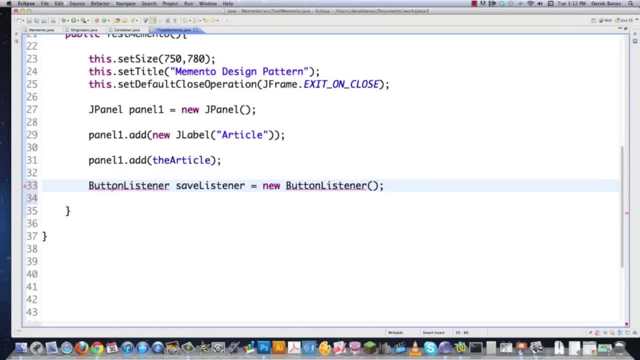 If you have any questions, just leave them down below. Sort of speeding through some of this stuff, because I've covered it so many times in the past. And then we're going to need an undo listener and a redo listener. These are just going to be buttons that are going to undo and redo. 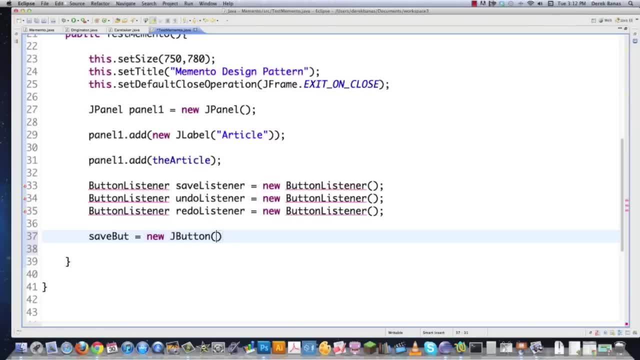 Save button is going to be equal to new J button And I want to put save on that button And then I just need to come in here and go save button. Add action listener, which is going to allow me to do certain things whenever the button. 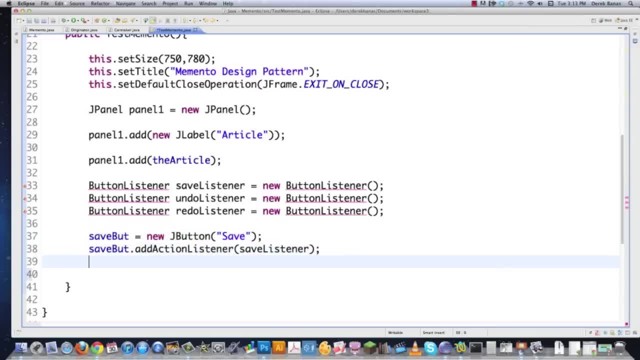 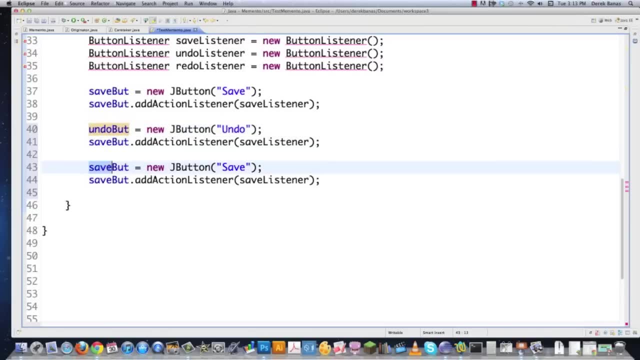 is clicked on, Then I'm just going to copy this: Do the same thing for redo and the undo button. So let's do undo here and make sure we save this as undo, And this is going to be redo. Just going to make the different articles pop up here on the screen. 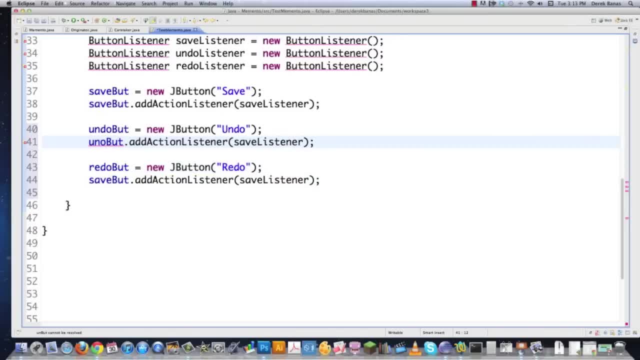 That's all it's going to do: Bounce back and forth through the different versions of the article whenever those certain things are popped through. here There's redo, And here we're just going to say undo listener And redo listener. And that's going to allow me to perform different events whenever those different buttons are. 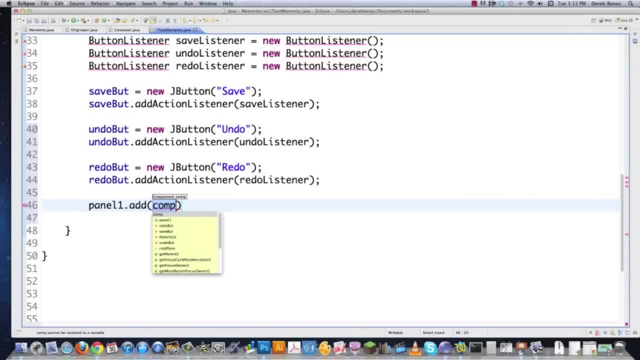 clicked on And then panel one. Of course we need to add our buttons, So save button, Copy And undo button, And redo button, And there's that. And then finally we need to add our panel. So say, hey, J frame, add my J panel. called panel one. 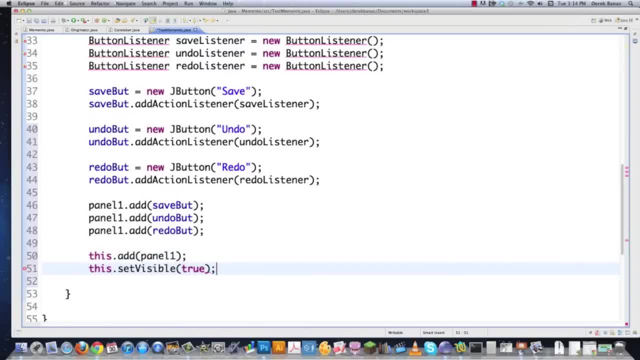 And then, after you get all that set, make my J frame show up, which is exactly what that does. That's kind of a review of use and swing- Always useful- And then I'm just going to throw in my J frame. And then I'm just going to throw in my J frame. 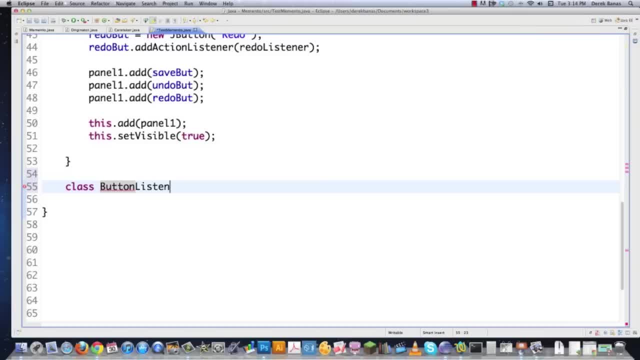 And then I'm just going to throw this class inside of here so that it will be able to access everything that I'm going to need: access to Implements, Action listener- And I'm going to go public void action performed And it's going to get an action event sent to it. 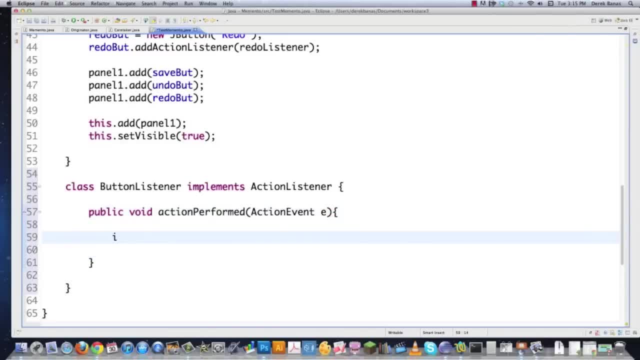 And I'm just going to call it E just to be boring. And then I'm going to say: if E gets source of the action that was triggered, well, this is going to say: did the save button trigger this action? If it did, well, I need to change. 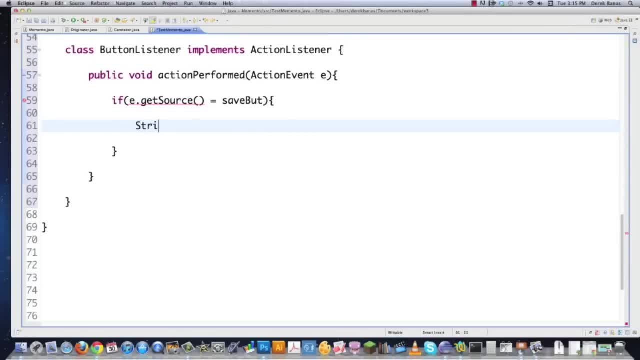 I need to change the value of my little text area on my screen, So I'm just going to create a string here. text in text area is what it's going to be called, And if I want to get the text in the text area, I just go the article, which is the. 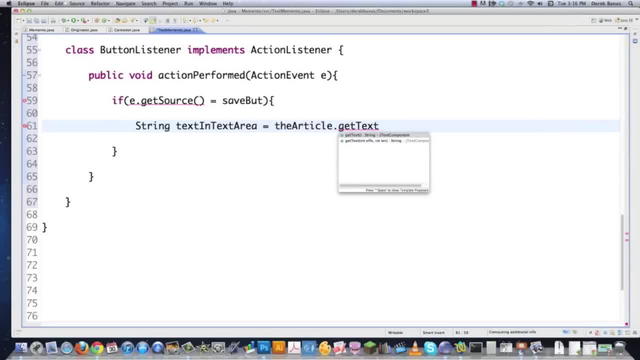 name for my J text feed text area and go get text. It's going to give me the current text stored inside of there And I'm going to go originator. So remember, I'm saving whatever is in the current text area on the screen to a memento. 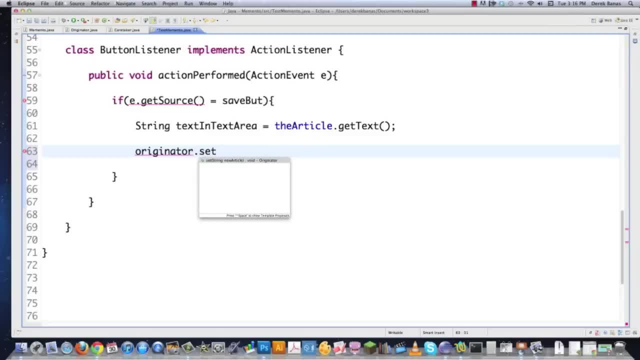 to a field inside of a memento. So then to do that, I need to call originator set and then go text in text area And this is going to save that to article inside of the memento object so that we'll be able to use it later on if we ever leave this area. 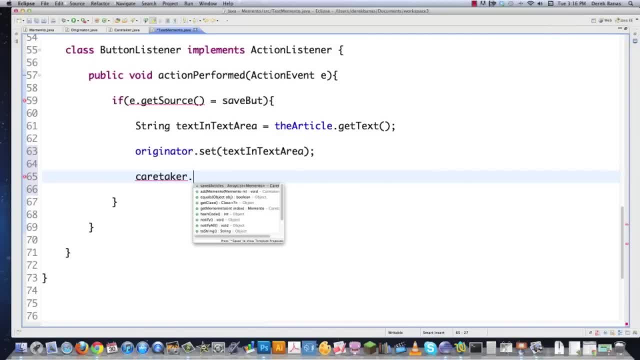 And then we got our caretaker. I need to add my new article to my array list or my new memento object with a new article and just go originator store in memento like that. And then, since I saved a new object inside of here, 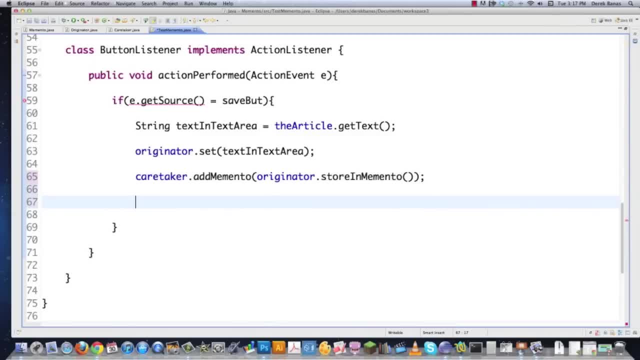 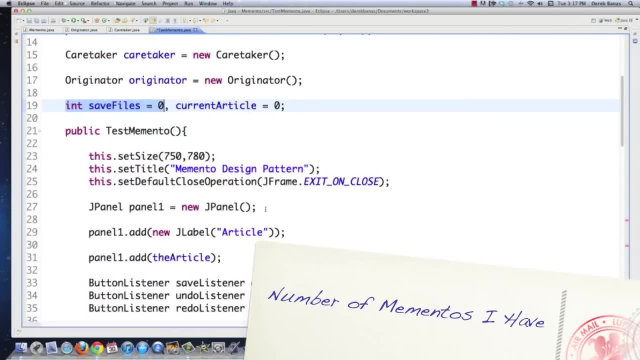 I want to increment my number of saved files, So I'm going to go save files. Remember, that's up here somewhere. There it is. See, this is going to tell me how many files I currently have saved. So that's important. 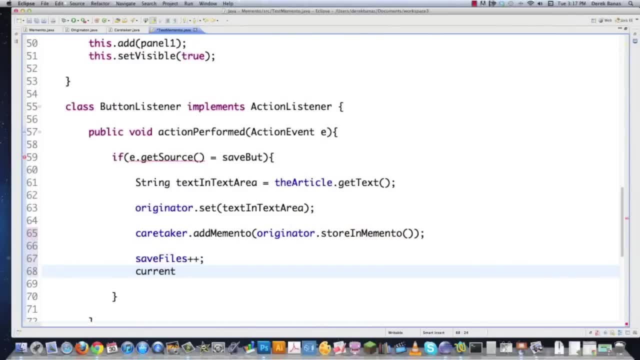 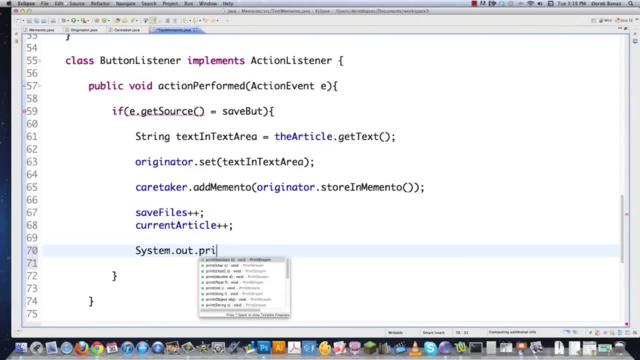 So just save files, increment that- And my current article is also going to have to increment because I just saved a new one inside of there- And then let's put out a little message. This is how I debug things all the time, by the way. 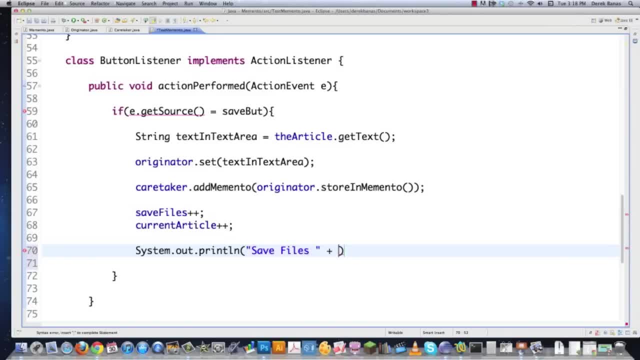 So save files. I just put a little note in here to print out the screen, What was just done, And this is just going to print out how many saved files I currently have for current mementos that I currently have, And then later on, whenever the undo buttons hit to the point that there are no more files to be brought up. 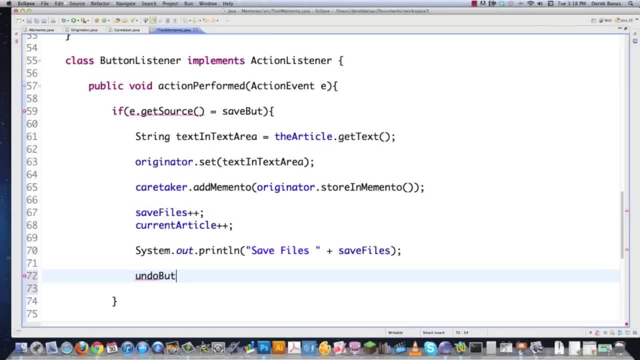 I want to actually disable that so that they won't be able to continue looking for memento objects that don't exist. So I'm going to go set enabled to true, because I just added a new one. So that's going to mean that I'm going to be able to undo and go back to my previous one. 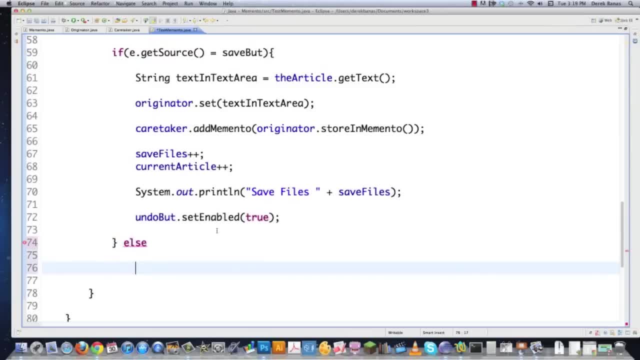 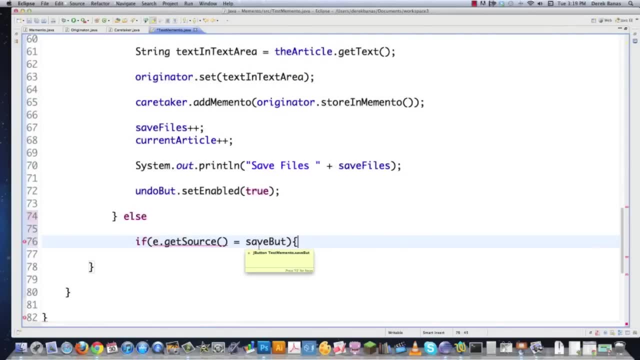 Think about that for a second, or leave a question below and you'll get it. And then I'm basically going to do the same sort of thing here. I'm going to check if the source of the click was done by some other button In this situation. I'm going to check to see if it was the undo button that was clicked. 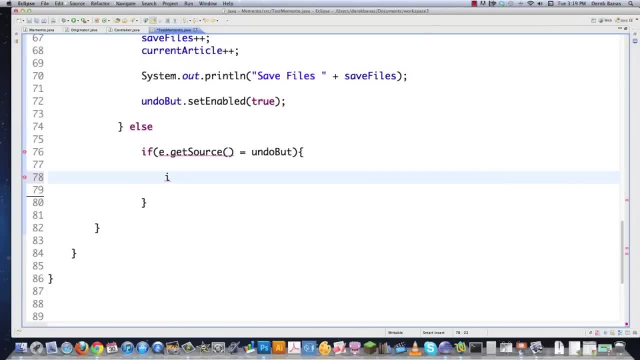 So undo button. And if it is, I want to perform a couple of checks here. I'm going to say if current article is greater than or equal to one. I want to make sure that I am not going to try to go to a memento object in the array. 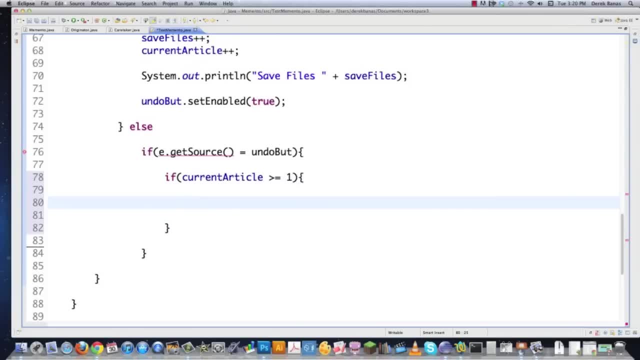 List that doesn't exist. So I want to make sure that it is going to have a value of one, so that the maximum value for current article is going to be zero Because the index or the minimum index for the array list is going to be zero. 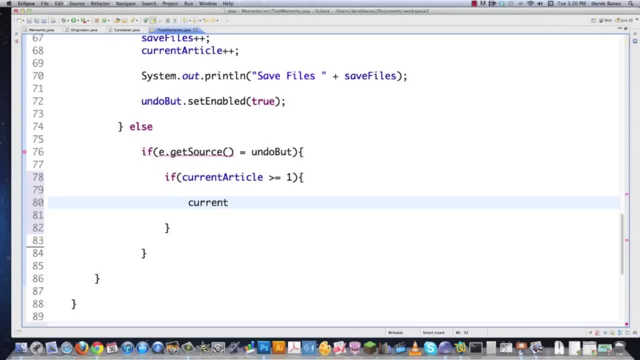 So I'm checking if it's greater or less than one, because I'm going to decrement it. So that's just a check to make sure I stay inside my array list. And then I'm going to go string- text box string And I'm going to get the current value for the article. that's going to go inside of the text box. 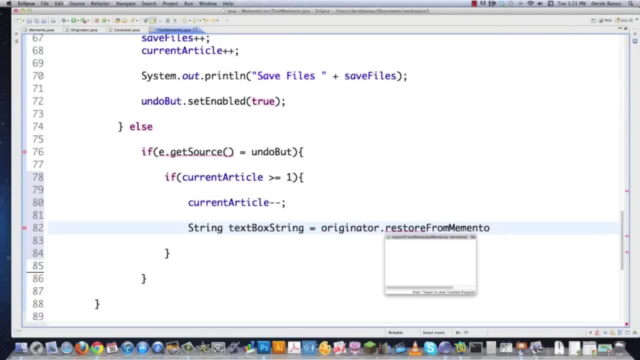 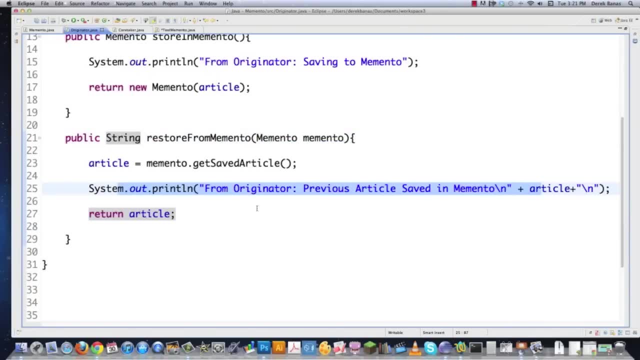 So I'm going to go Go. originator restore from memento. We can look at this thing. Here's originator restore from memento. I'm going to pass it a memento object And it's going to kick back the article that is saved in the memento. 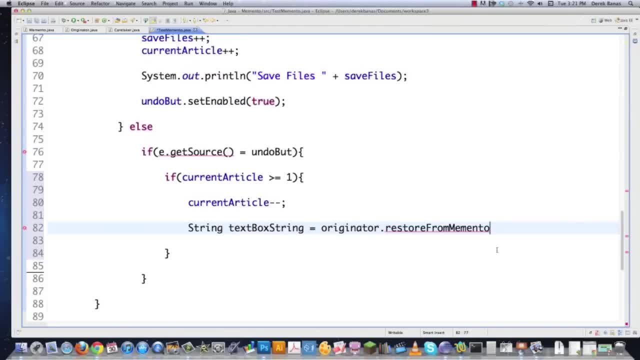 See, that's what it does, So let's bounce back here. Restore from memento. Well, I'm going to need to go. Hey, caretaker, I want to get the current memento And because I decremented current article, that's going to get me the index inside of the array list for the last one of those guys. 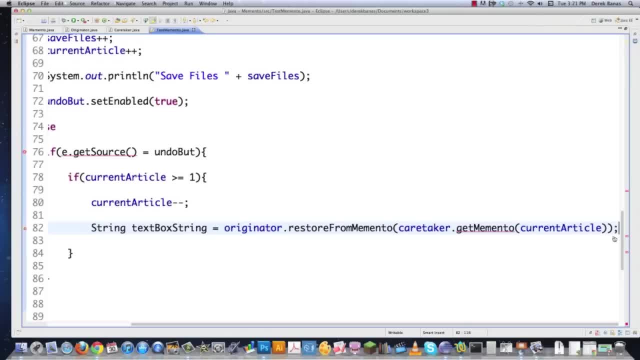 And then my men say: get rid of that, I'll save that. Jump back over here, Memento. See, that went away, That little error message. Sorry, when I improv a little bit I occasionally make a couple typos. 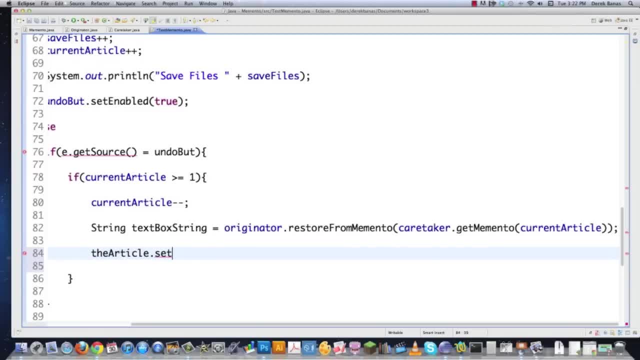 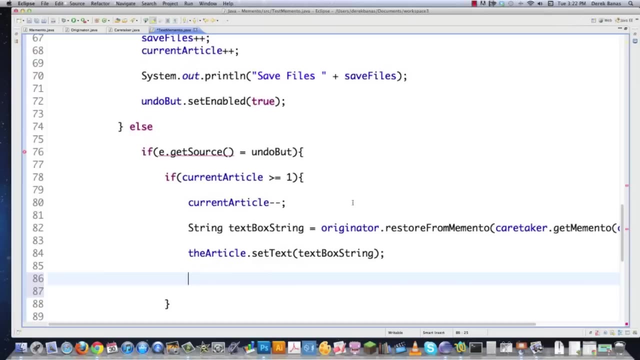 And then I'm going to say the article which is the J text field. I'm going to set text to whatever the article is stored in that memento object, like that. And then also remember we're doing this thing where we're enabling and disabling the buttons so that we don't accidentally call for an index that doesn't exist in the array list. 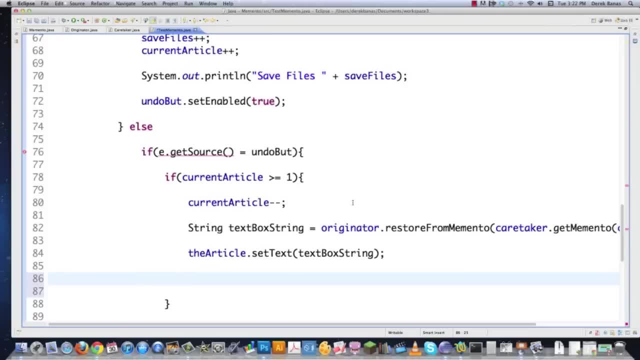 Since we start at zero and go up to the maximum number of files that are saved. Well, since we did an undo button here, I want to make sure if redo button was grayed out, I want to set enabled to true Because since undo was pressed, that means we're going to be able to redo. to go back to the previous one: 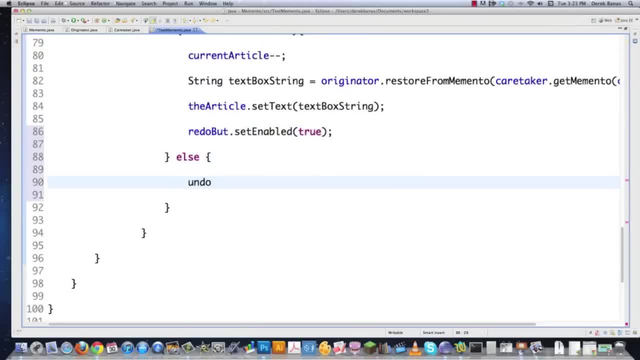 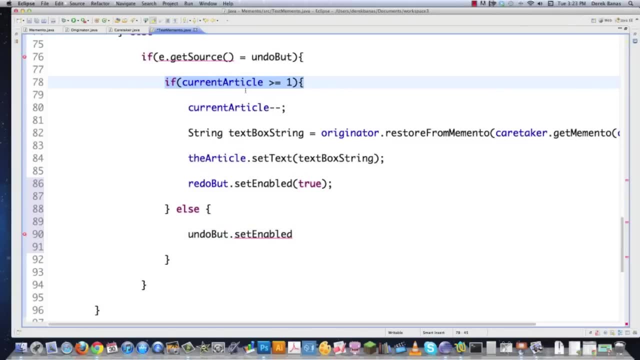 So that's what I'm doing there. That's neat. Else, I'm going to say undo button set enabled. That means we tried to go to see if we got to here, But current article was not Greater than or equal to one. 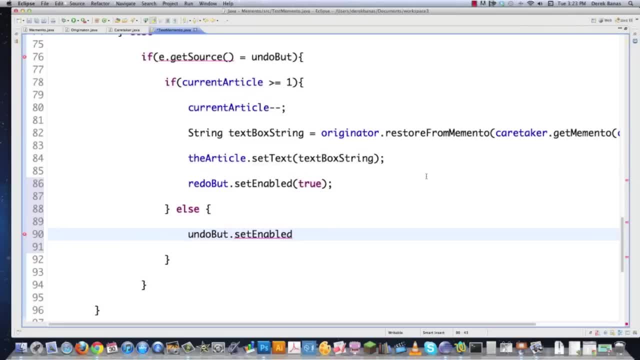 That means we were about ready to fall out of our array list and call up an array list item that didn't exist, which would trigger errors and cause all kinds of havoc. So what we're going to do is set enabled for the undo button to false, so that we don't have to worry about trying to access an array list item that doesn't exist. 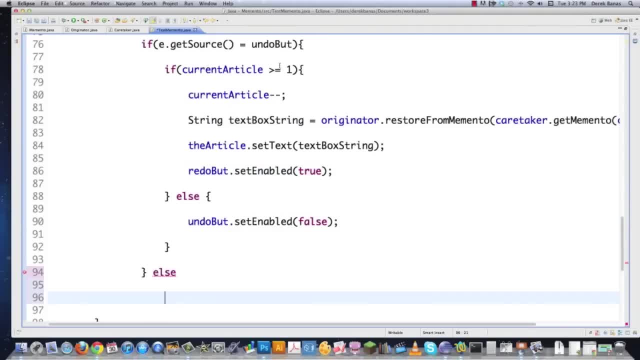 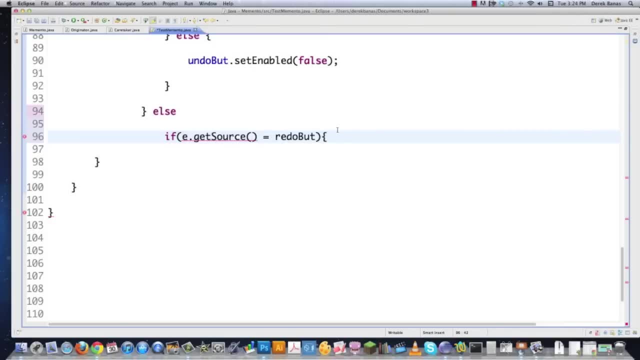 And then down here we're going to go else and then we're going to do another if statement. So we might as well just copy that right there, Paste that in there, And here we're going to check if it's the redo button that was clicked on. 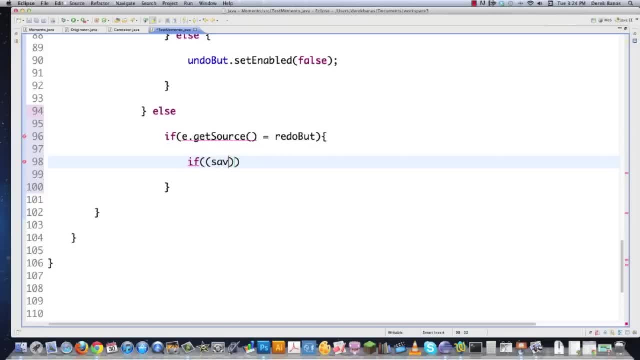 And then, In this situation, we're going to check save files, because that's going to tell us the total number of files that we have in existence, that we've created, And I'm going to subtract one from that and make sure that current article is greater than one minus the total number of files that we have saved, because we don't want to try to bring in a new save file that doesn't exist. 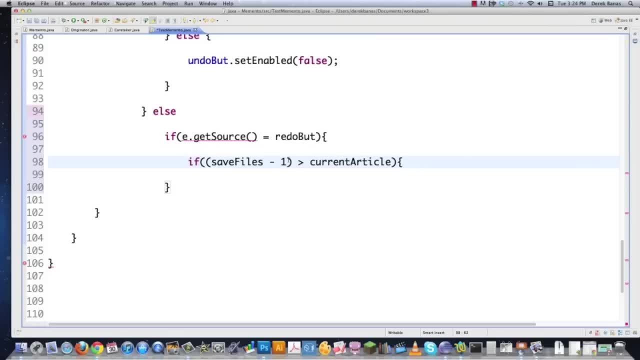 And the reason why the negative one is there is because the index, of course, starts at zero. So now that we Are able to do that, we're going to increment the current article so that we are using a new article, and then get the newer article saved and display it inside of our text area. 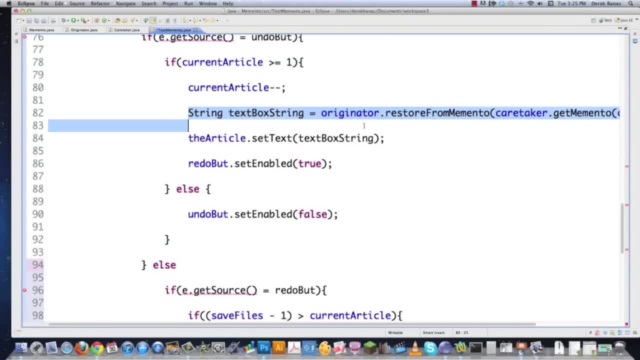 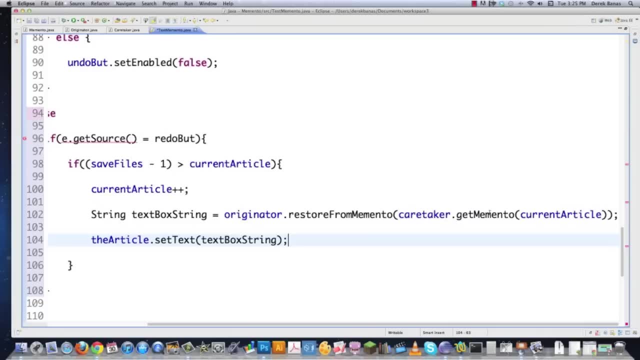 And we're going to do that pretty much in exactly the same way that we did before. So let's just copy this, paste that their text box string, and then we're going to call originator just like before. Restore for memento and get memento. 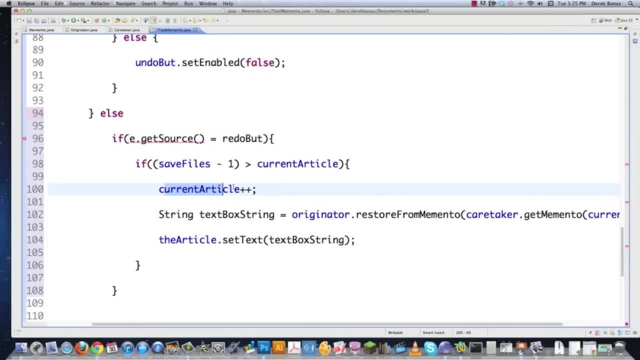 And then this guy is going to be exactly the same, because we incremented the current article. So we're just bouncing through that array List. That's all that's going on here. And then we're going to set the article, which is the J text field. 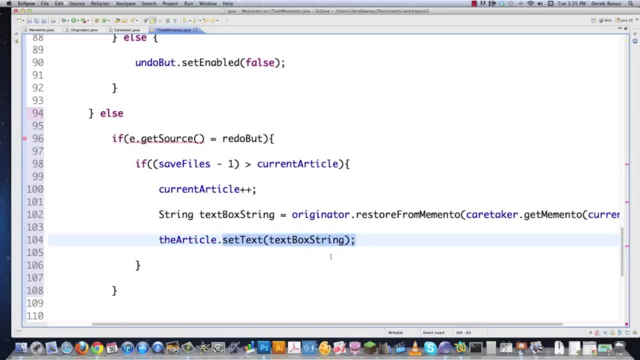 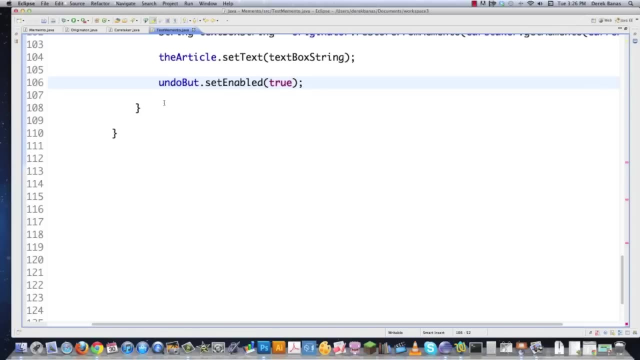 It's going to show up on the screen using set text by putting that information inside of there And because we did hit redo button. what does that mean? That means our undo button is now going to be usable. So we're going to make sure that our undo button shows up as true and then else. 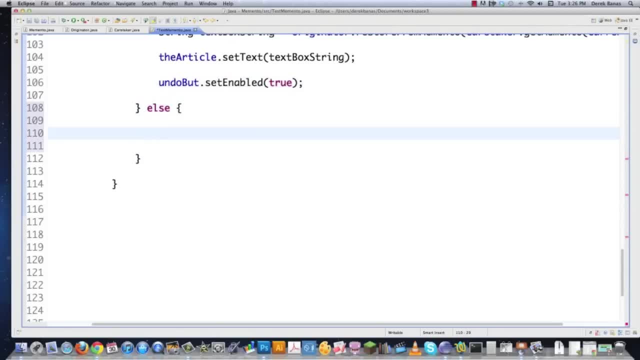 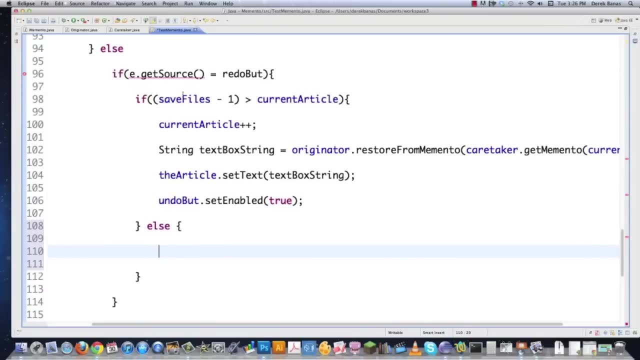 And when will it get to this else? It'll get to else whenever we hit the redo button, Which means we're going to advance upwards into the future in regards to changes that we've made to article. And what does that mean? That means redo button set enabled should be set to false so that it's grayed out and can't be clicked on anymore. 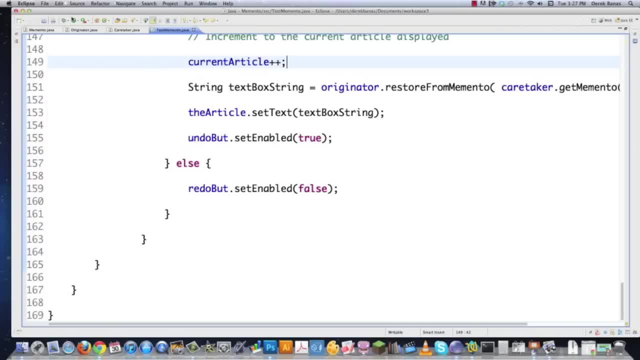 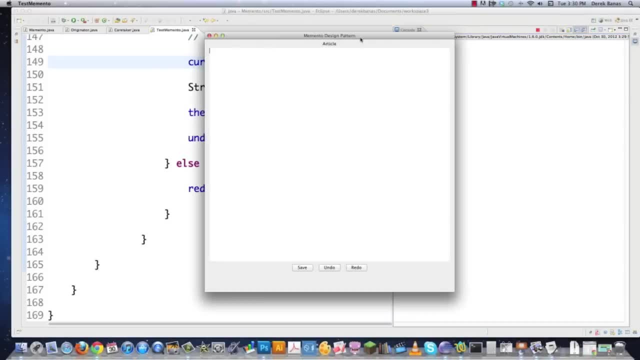 which would cause all kinds of havoc, And file save that And now let's check it and see if it works. So let's run it, And I'm also going to have my console over here on the right side of the screen So you'll be able to see what's going on over there. 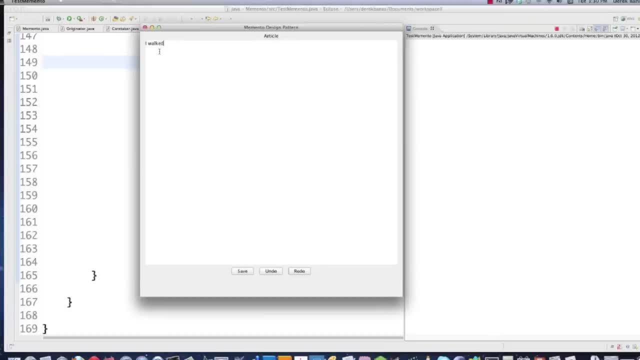 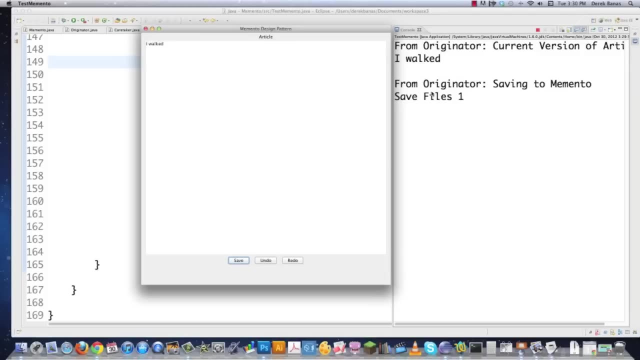 So let's say, I walked was just quite simply What I typed in right there. I walked and I'm going to hit save And you can see from originator. current version of article is: I walked and from originator: saving to memento. 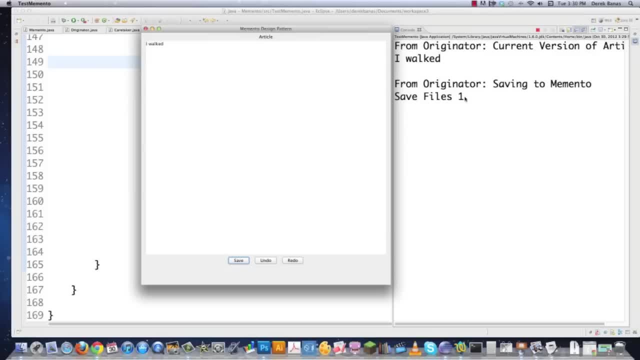 which is going to save this new field data over to a new memento object And then save files means I have one new memento object inside of an array list. Okay, then I could say: I walked down the street like that: Real, real, real, simple. 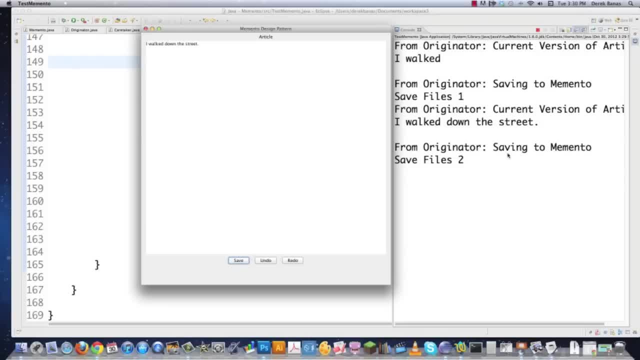 And then hit save And now you can see current version is. I walked down the street from originator And now we have to save files. And then I could say: and I saw something like that and save that And you can see everything's updating over here on the right side of the screen. 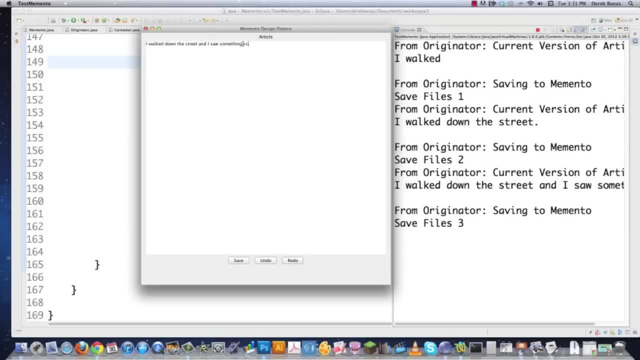 And then, finally, I could say I saw something scary and real simple and hit save again. And there you are. You can see, I walked down the street. I saw something scary. Now let's show how all of the undo and redo buttons work, which are down here. 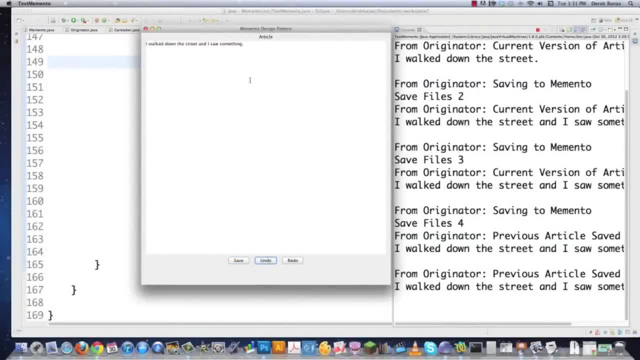 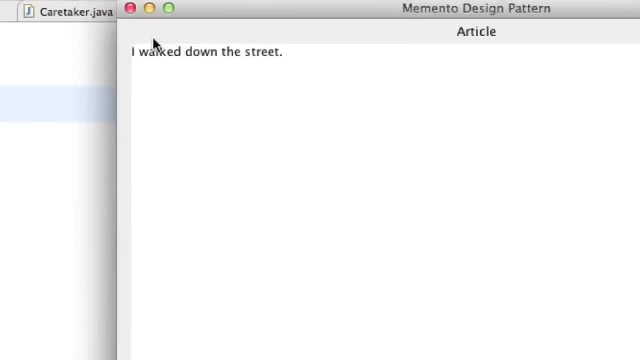 I just been hitting save over and over again. So if I hit undo, you're going to see I walked down the street and saw something You can see the scary part jumped off of there And then if I hit undo again, you can see it changes to: I walked down the street, which is another previous version.